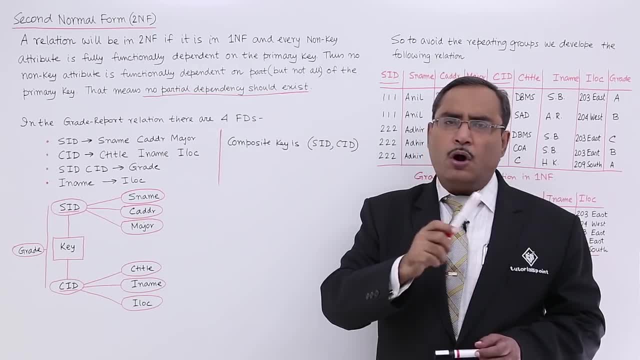 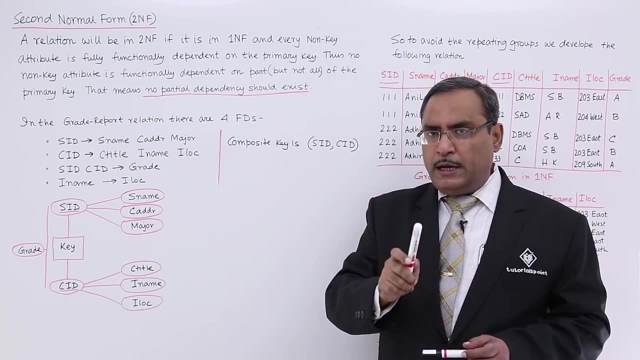 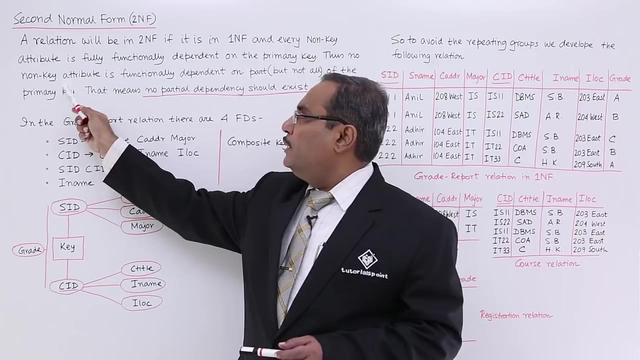 those will be which will be participating, will be known as a prime attributes or key attributes. So it is telling that all the non-prime attributes or non-key attributes should be dependent on, functionally dependent on all attributes in the primary key. Thus no non-key attributes is functionally dependent on part but not all of the primary key. That 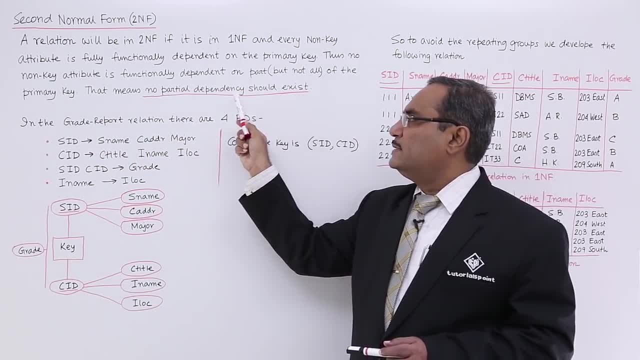 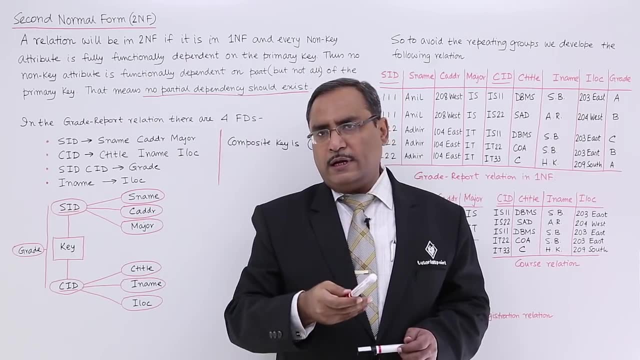 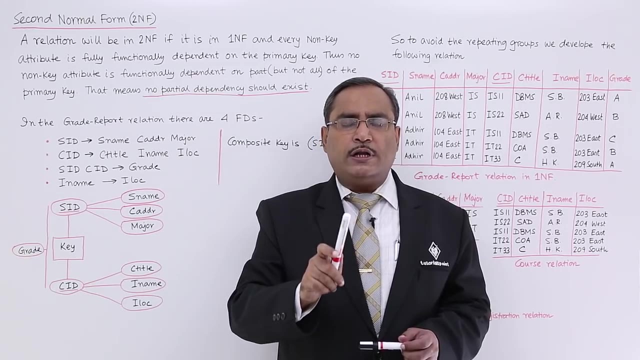 means no partial dependency. So that is why I have put underline here. it is very important. So let me discuss partial dependency once again for your better understanding. Partial dependency means some of the non-prime attributes are fully functionally dependent on some of the prime attributes, but not all. 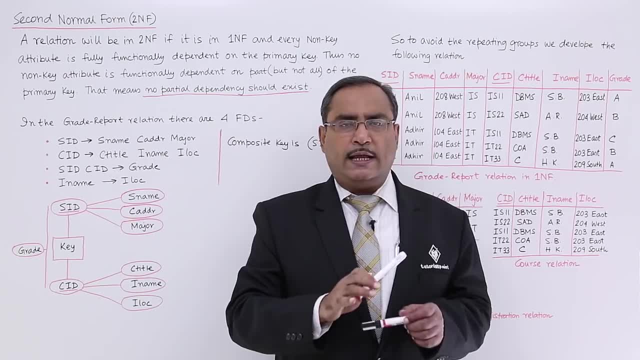 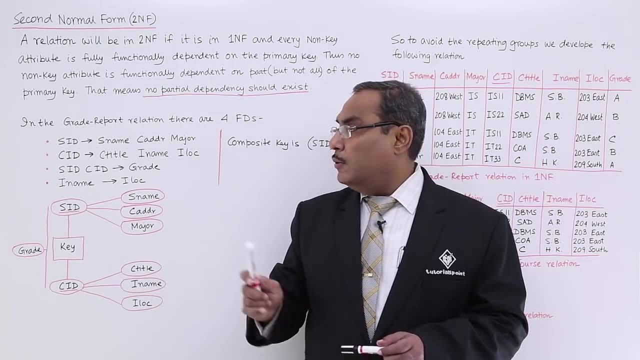 So if such situation occurs, then we shall say that the relation is not in 2NF, and another condition is that the relation must be in 1NF. Now let us go through one example. So this is the relation, the name of the relation. we 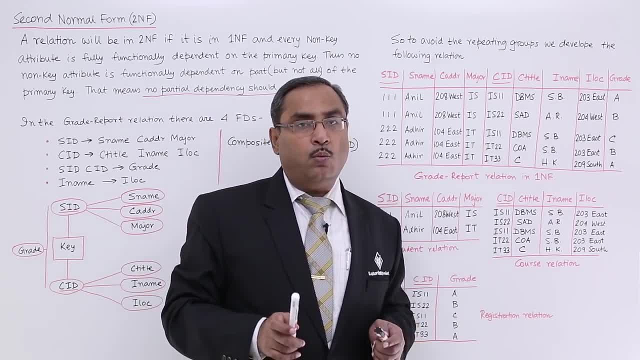 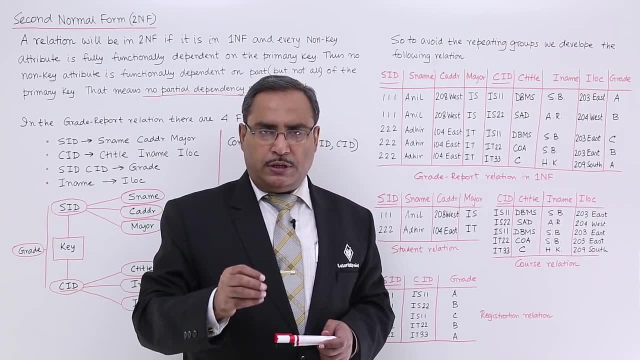 have given is grade report relation, which you did in our 1NF. So this relation is having the student ID and the course ID as the primary key. that means composite key. A primary key consisting of more than one attributes would be known as a composite key. 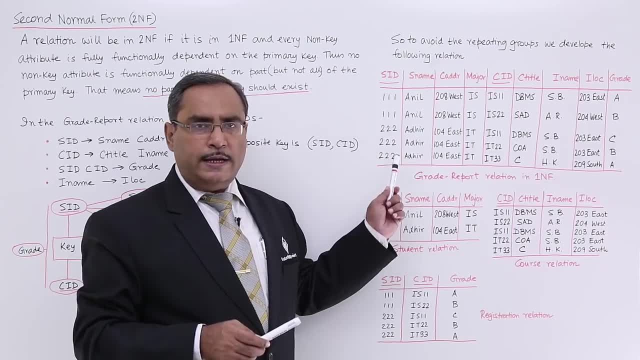 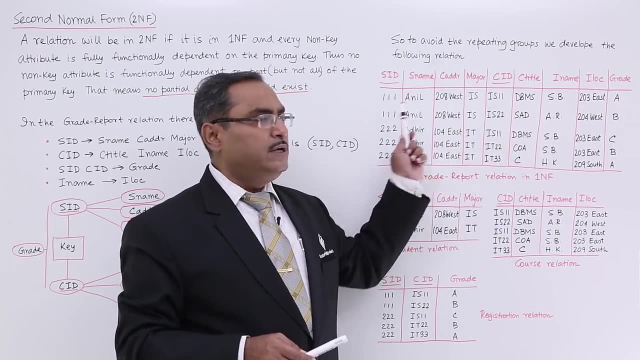 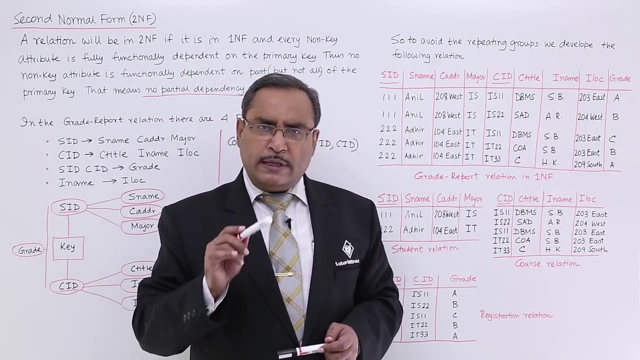 So here you see, only roll number or student ID cannot identify tuples uniquely. Only course ID cannot identify tuple uniquely, but this combination is unique. So that is why student ID and course ID will be known as the composite key or primary key. We know that whenever there 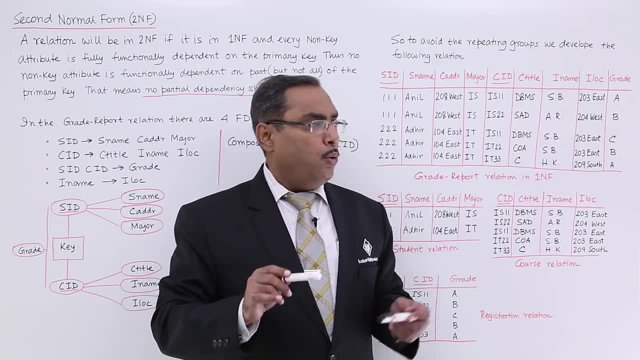 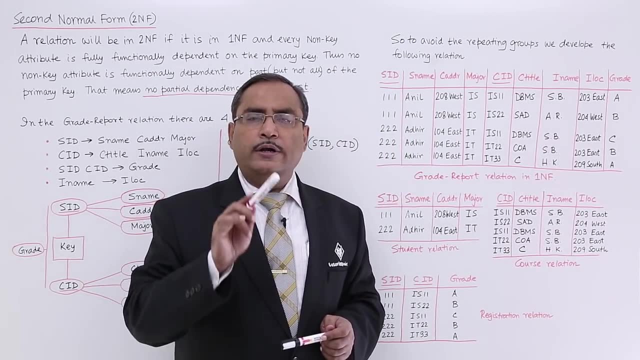 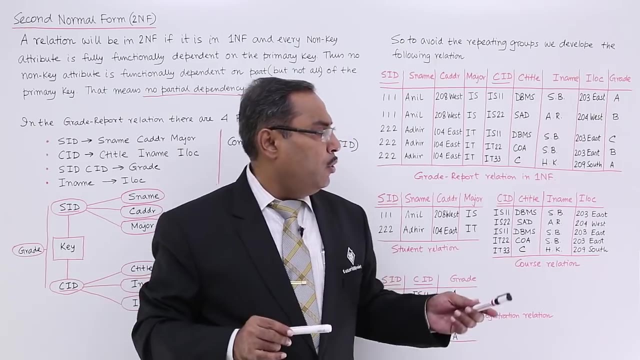 is a primary key whenever there is a prime attribute. while inserting any kind of record to this particular relation, I cannot leave blank or null to the prime attribute. I must be putting some, not null, value to the prime attributes and that is mandatory. This relation is suffering. 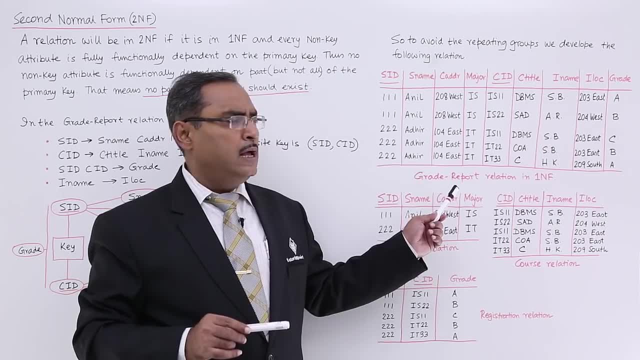 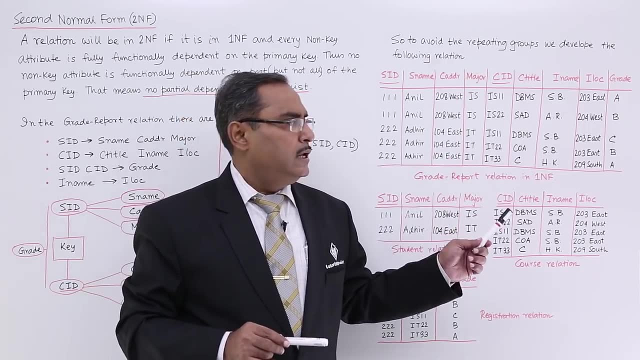 from anomalies, Why this relation is suffering from anomalies? Because it is not in 2NF. Why it is not in 2NF? I shall discuss that one. Let me tell you the anomalies. at first, Anomaly number one, that is the insert. anomaly Here: let us suppose the university who 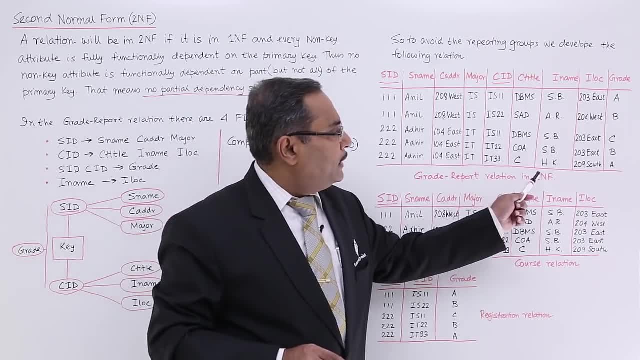 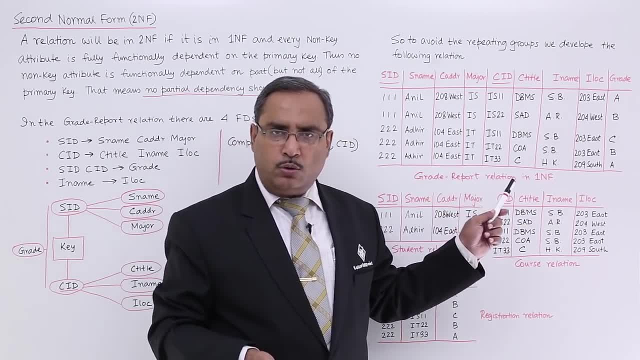 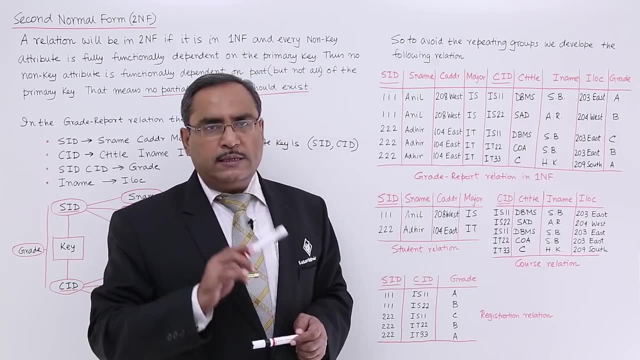 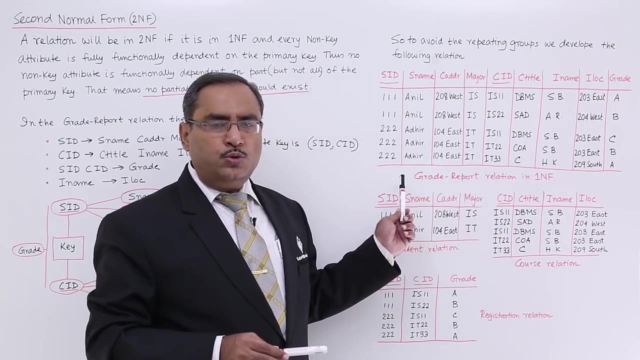 but as no student has taken admission to that very course right now, so the student ID will remain null. so the course entry cannot be made here. So that is our insertion anomaly, Let us go for the deletion anomaly. Let us suppose there is a single course and only one student has taken admission to that course. 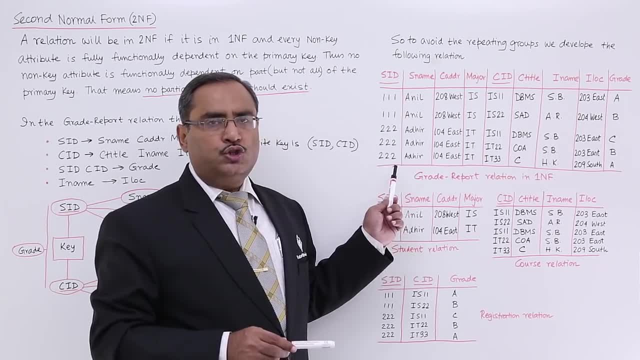 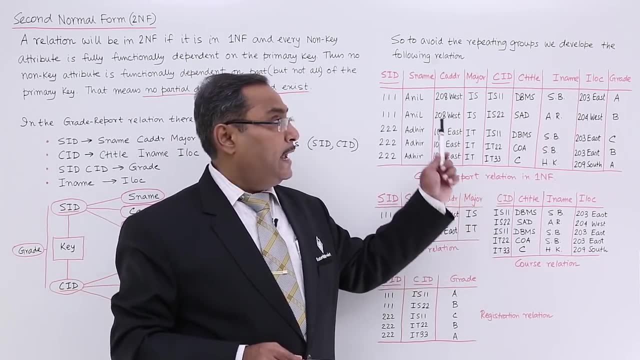 Due to some reason, this student is leaving this university, so the respective student ID is getting void and null. So I cannot keep this record intact here, Because I cannot leave one prime attribute filled up with a null value. So what is happening in this deletion process? 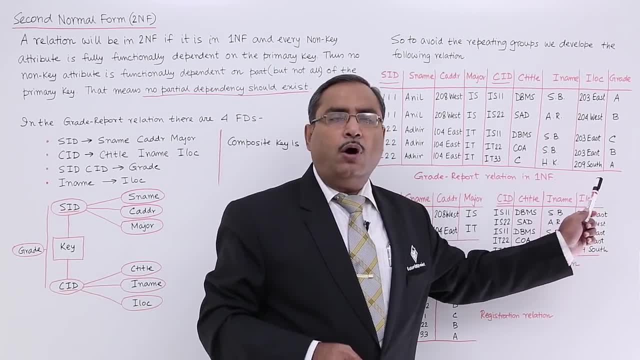 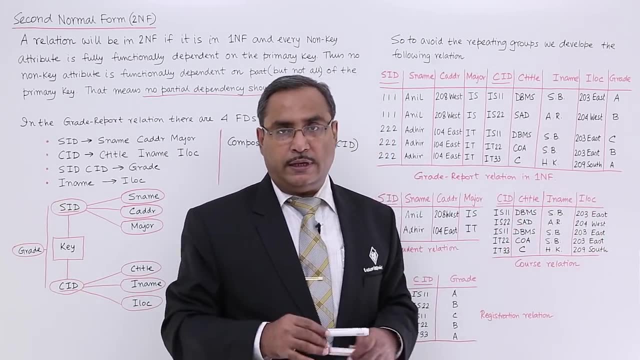 In the meantime, we are deleting the new course details or the course to which only one student took the admission, So that course details will be lost along with the instructed information and everything. So that is our deletion anomaly. Let us go for the updation anomaly. 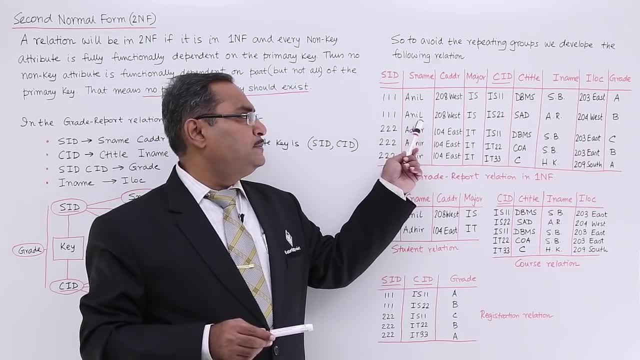 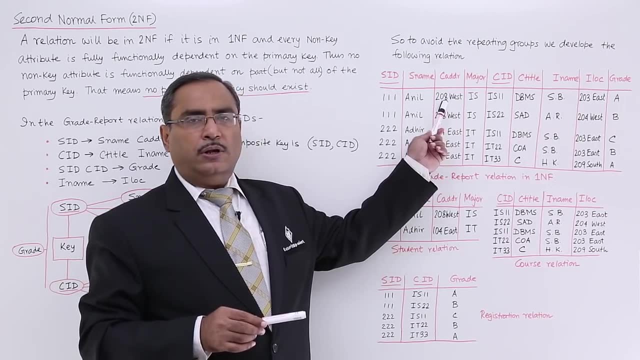 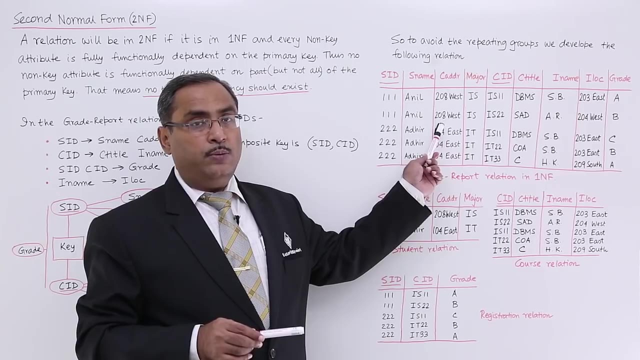 Anil has changed his address. But, Anil, this particular address has occurred for twice. Let us suppose while doing updation, due to some means, this particular address, one of the instances have got updated and another instance have got not updated. So that is why we are leaving the system in some inconsistent state. 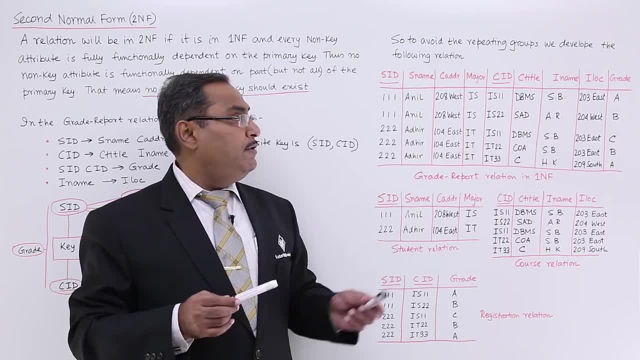 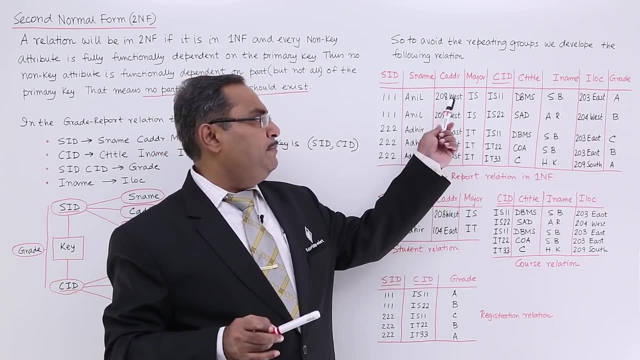 So next time, if I execute one query which will give me the address of Anil, I will be getting two answers, and that is not consistent. Always remember: whenever there is some same data is getting replicated for the multiple number of times on the database. 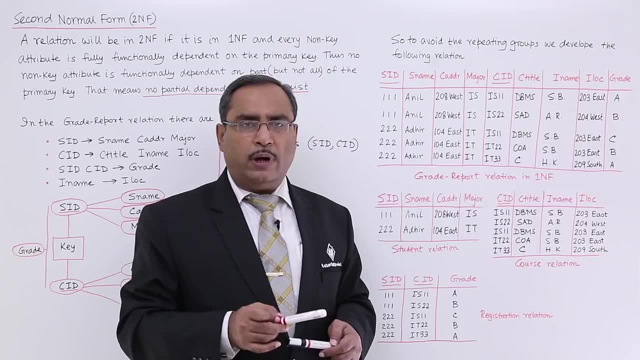 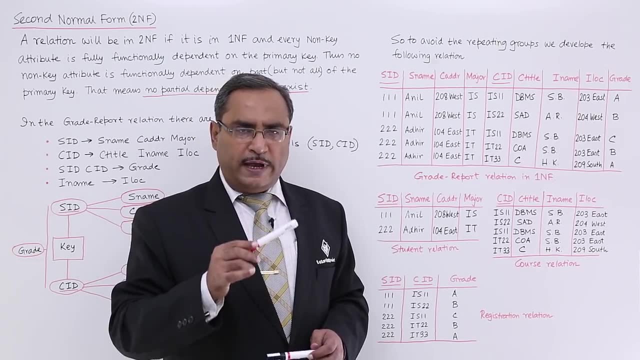 it occupies more space. That is the point number one. Second point is that data redundancy is there, And the third point is that there is finite probability of execution of partial updation leaving the system behind in inconsistent state. So that is our update anomaly. 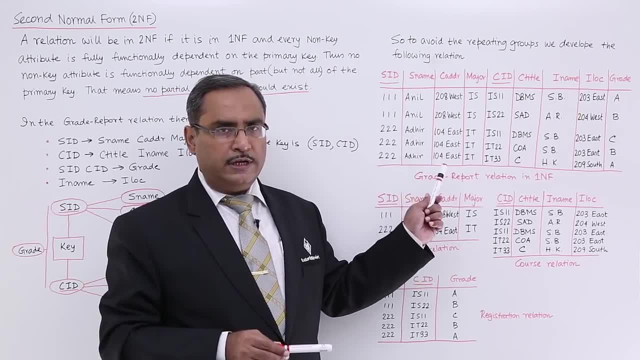 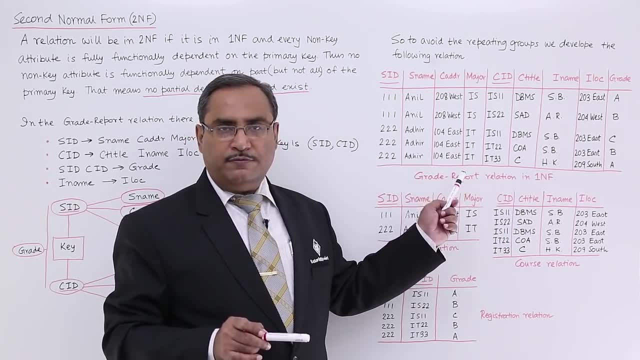 So all the three anomalies we have discussed on this particular deletion. So this relation, yes, good enough, We can easily work with the read-only mode, But in practice if you go for insert-delete, So we can easily update type of write operations on this relation. 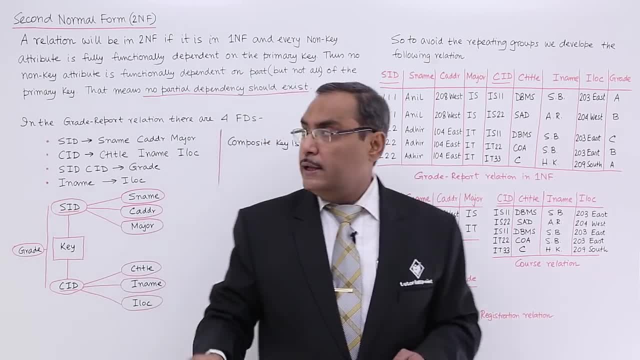 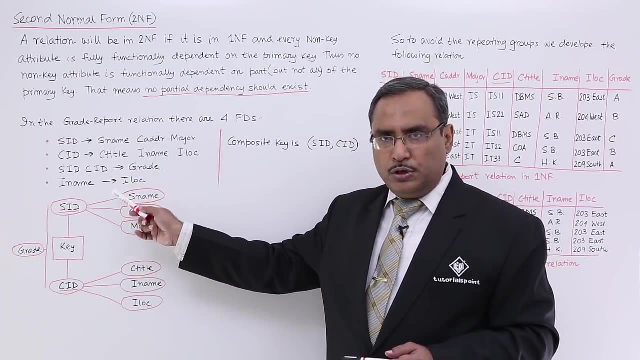 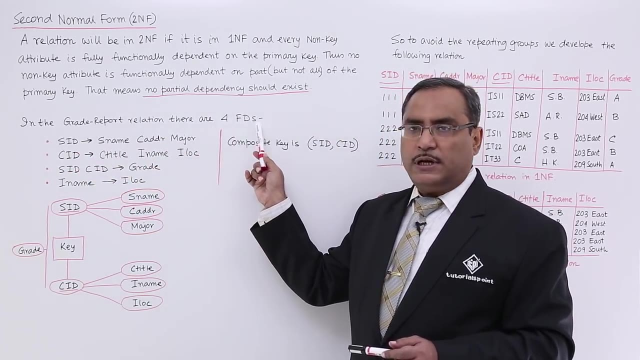 It is not possible. Why it is not possible? Okay, Judging all these values in this particular relation, we have come to this particular conclusion that this relation is having four functional dependencies. So in the grade report relation there are four functional dependencies. 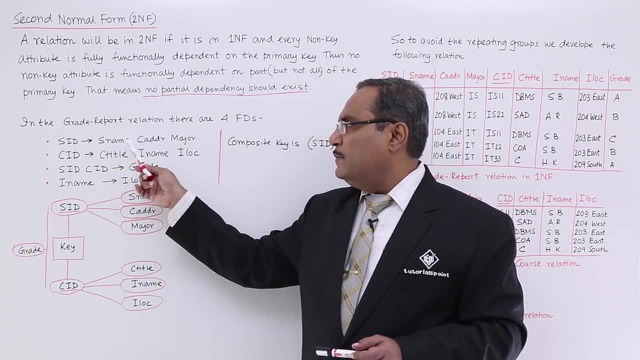 First one is: student ID determines student name, campus address and major Course ID determines student name. Course ID determines student name, campus address and major Course ID determines student name, campus address and major Course ID determines student name, campus address and major. 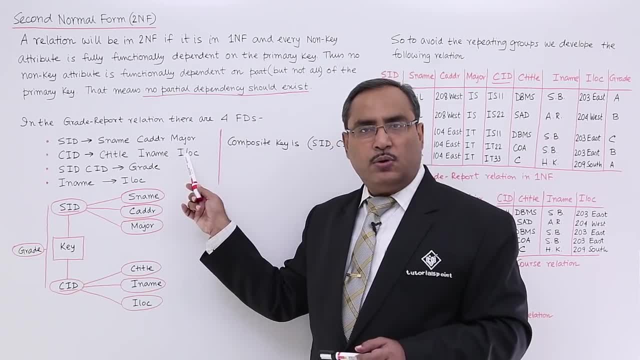 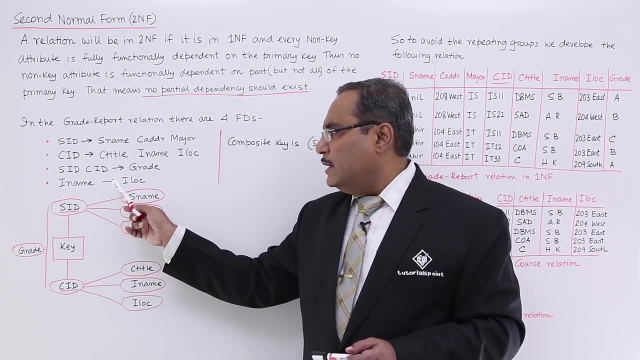 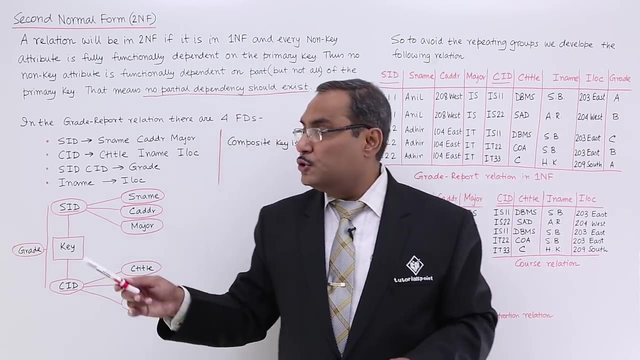 So it determines course title, instructor's name and instructor's location. Student ID- course ID determines grade And the last one is instructor name- determines instructor location. So, looking at these values and looking at the relationship between the attributes, we have reached. 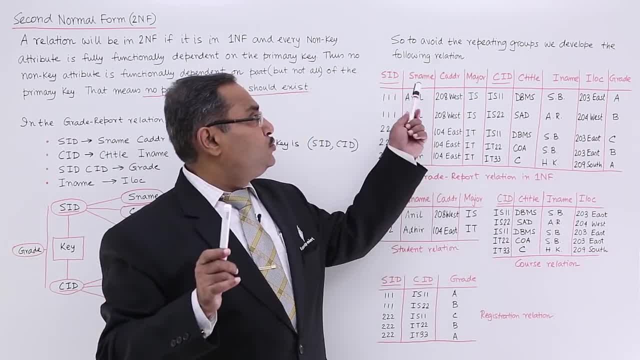 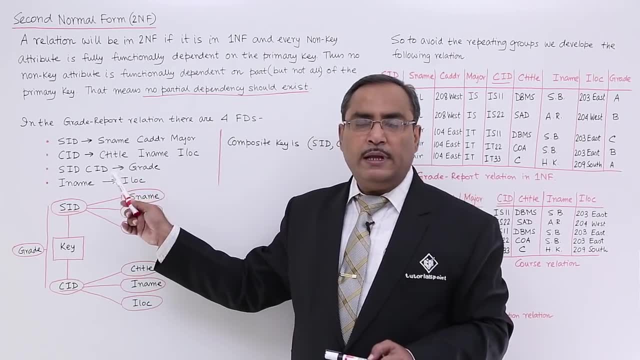 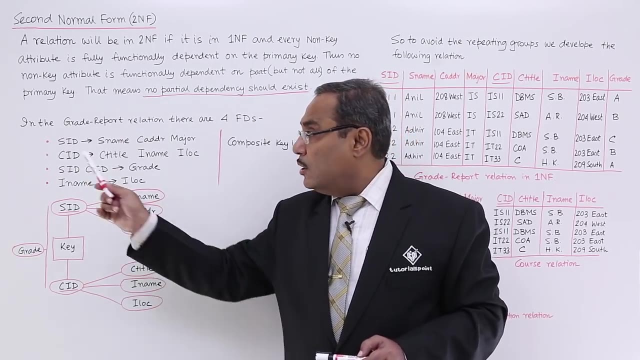 to these four functional dependencies. Here this student ID and the course ID is a primary attribute, primary attributes. So as a result of that, here we are observing partial dependency because only only student id, not all, not course id. student id, only student. 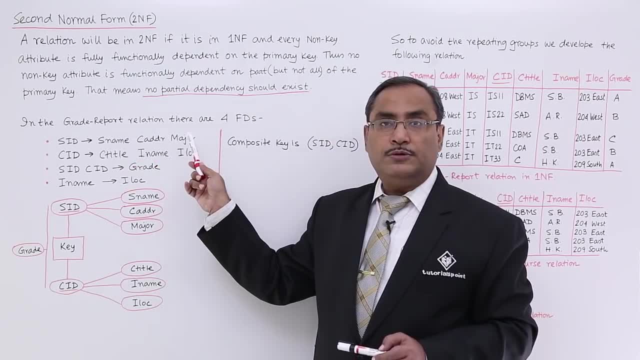 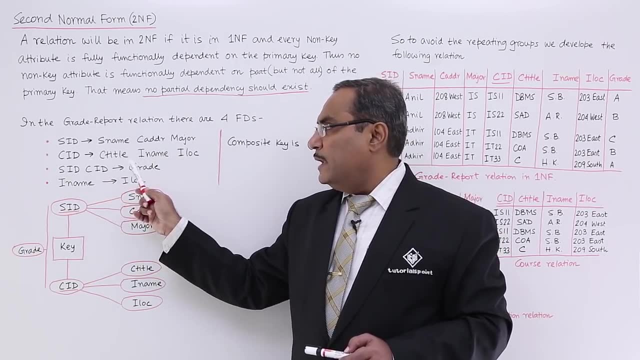 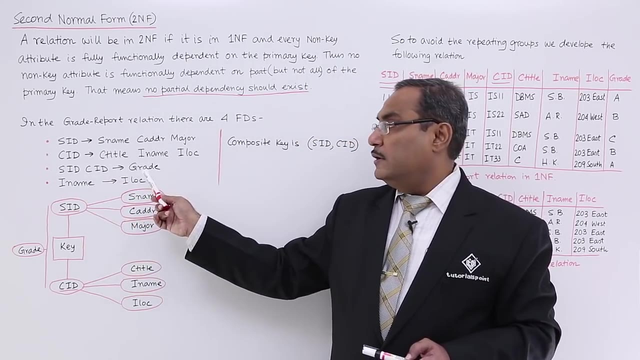 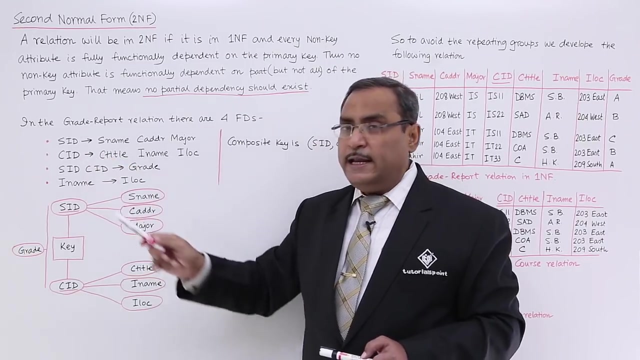 id is determining some of the non-prime attributes. only the course id is determining some of the non-prime attributes: student id, course id determining grade. that is quite obvious because there is a primary key, so it will determine the respective non-prime attribute. but this two production, this two functional dependencies, it is there indicating that the 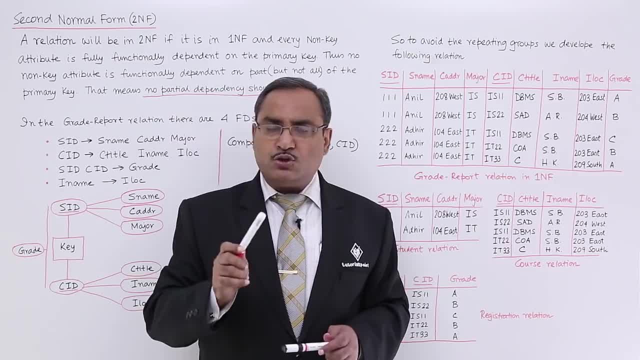 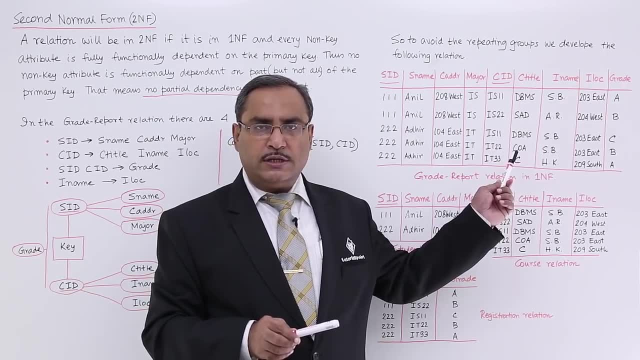 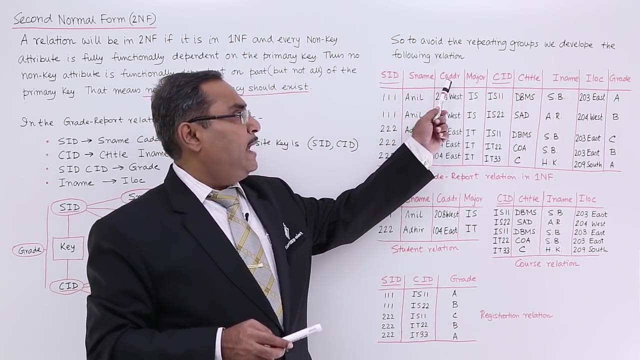 relation is having partial dependency and that is why all the three anomalies are there. so let us split this relation into multiple relations so that we can bring it into the 2NF. so student id determines student name campus at this major we are, we are having the first functional dependency here. depending on that, this student relation has. 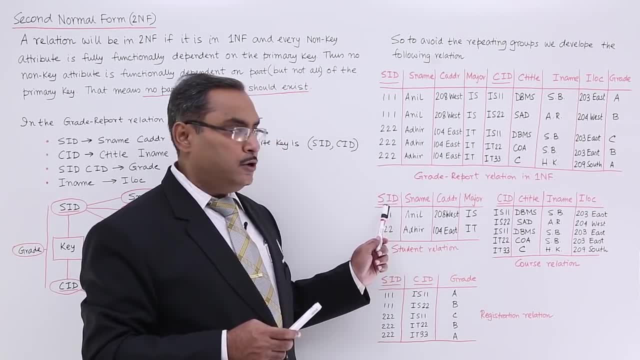 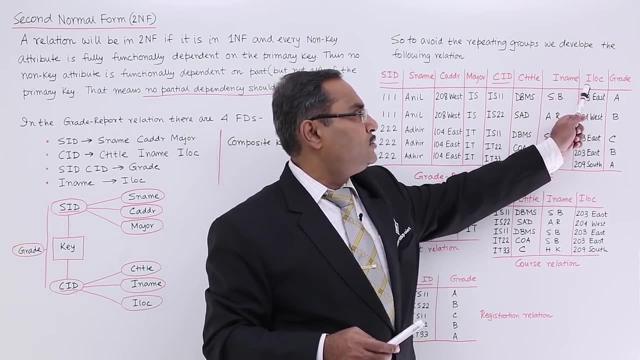 been х equal to the teacher's name, which of course is not needed anymore. 2NF has and been formed, so here student id is the prime attribute. next one we had course id determines course title. course title, instructor's name, instructor's location. so, depending upon the 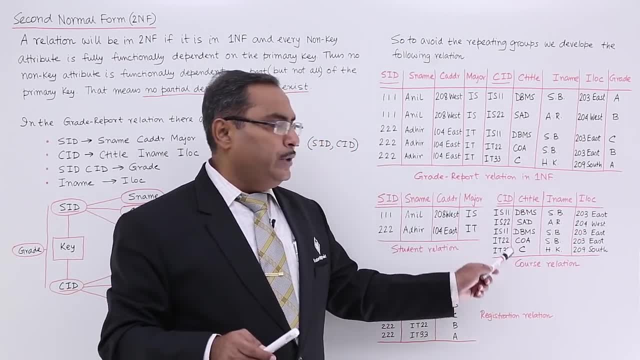 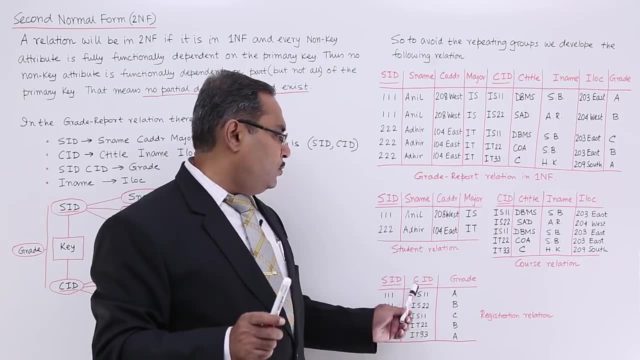 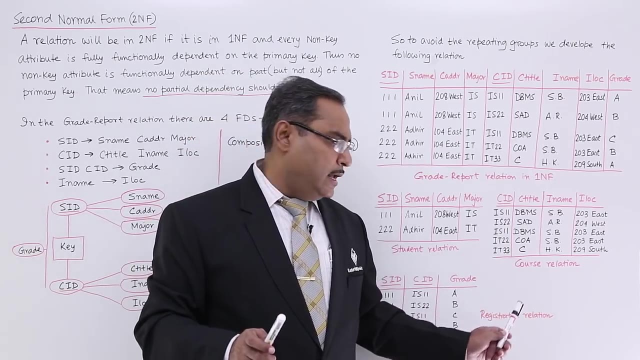 second, functional dependency. we have formed this particular relation with the name course relation. and the third one was student id course id determines grade. so student id, course id determines grade. so that is our registration relation. so we are having this student relation, course relation and registration relation. so this is our three splitted relations where 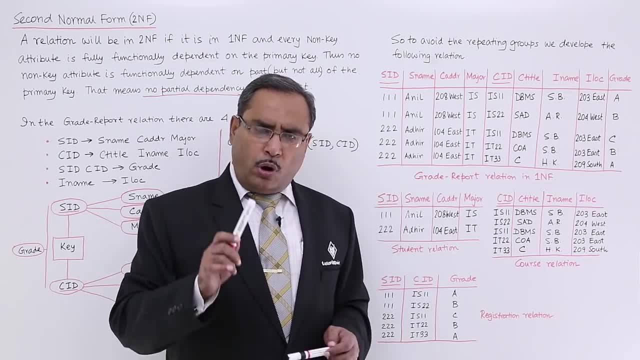 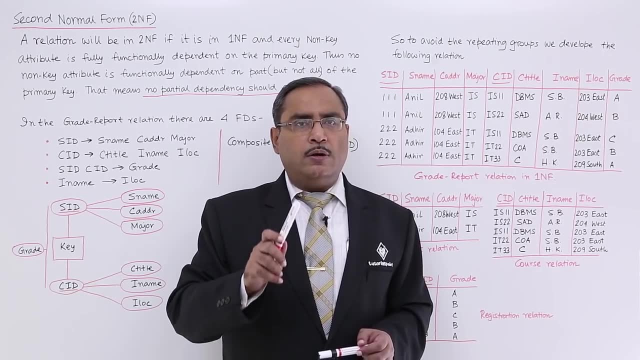 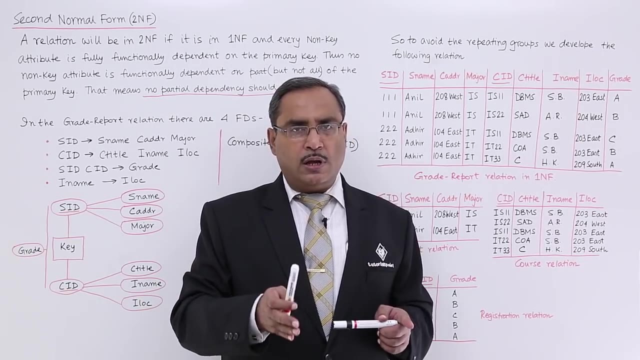 insertion, deletion, updation anomalies have got result. always remember, if the primary key is not a composite key, that means if the primary key does not contain more than one attributes, then the relation will be always into nf. that is no doubt because there is no chance of having any. 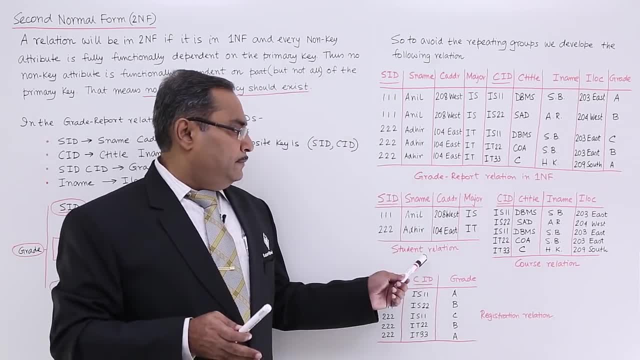 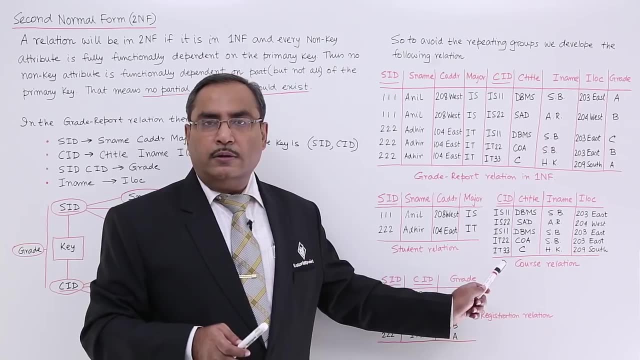 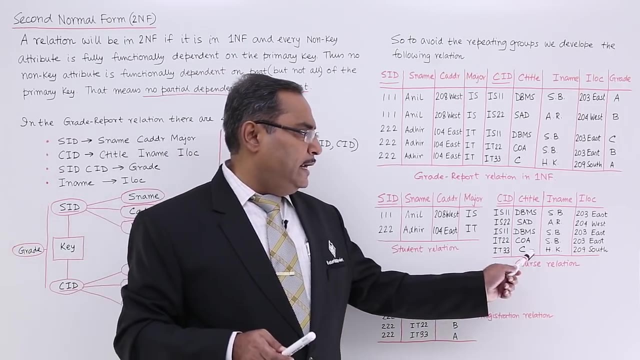 kind of partial dependence there. so this is our student relation, this is our course relation and the last one is our registration relation. in this way the anomalies have got result. let me show you. at first we are going for the insertion anomaly. new course has been introduced so i can put a tuple there with. 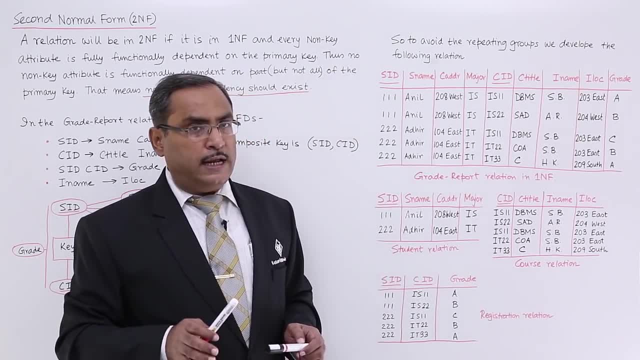 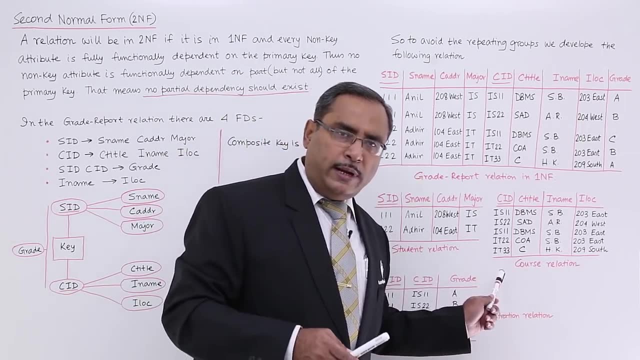 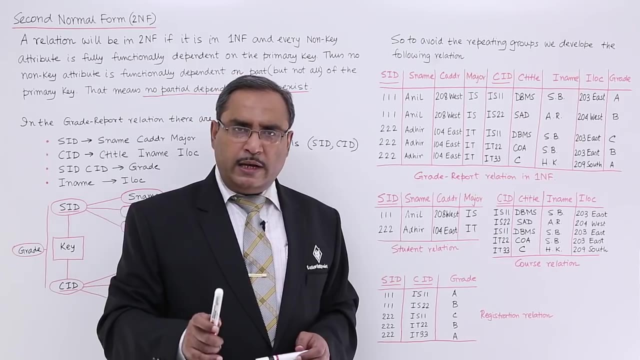 the course id and other details, but no registration has taken place yet. that is not a problem because course is having a separate relation where we can keep multiple new courses where no registration has taken place yet can be inserted. so insertion anomaly has been solved. updation anomaly. 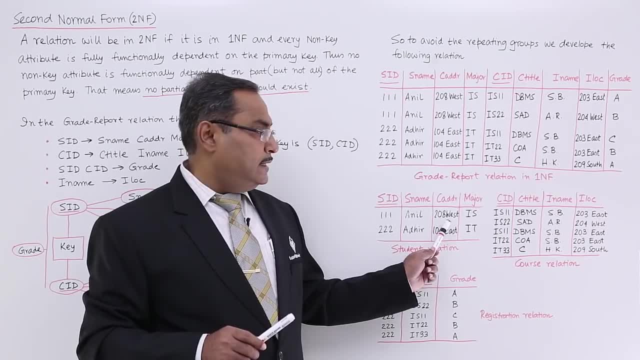 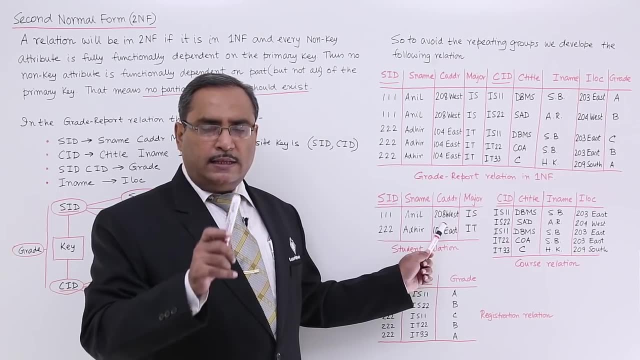 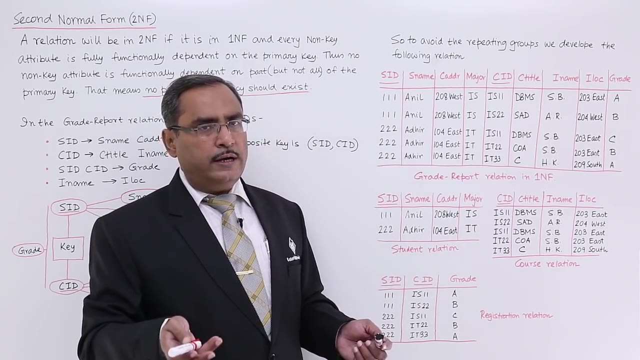 o'neill's address campus address is their mentioned in one place only. so if o'neill changes his campus addresses, in that case that respective updation cannot be partial updation, because only one instance is there, so all is. there is no data deep in if there is no data redundancy, data inconsistency. 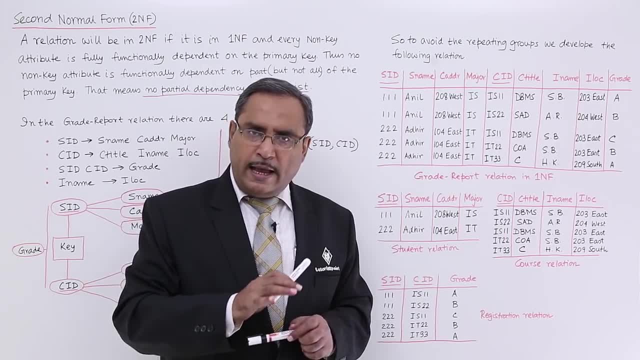 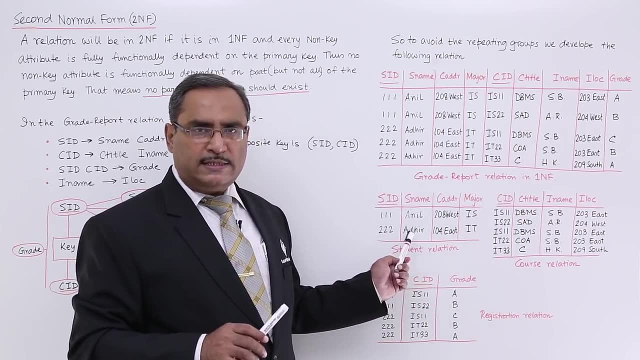 cannot come during updation, So updation, a total updation of this interior column is defined. form or data lock and order of declarable update anomaly has been solved. the last one is the deletion anomaly. there is one course to which only one student has taken admission and the student is leaving the university. then what will? 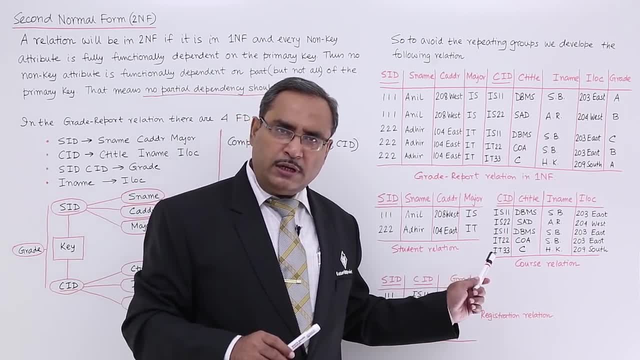 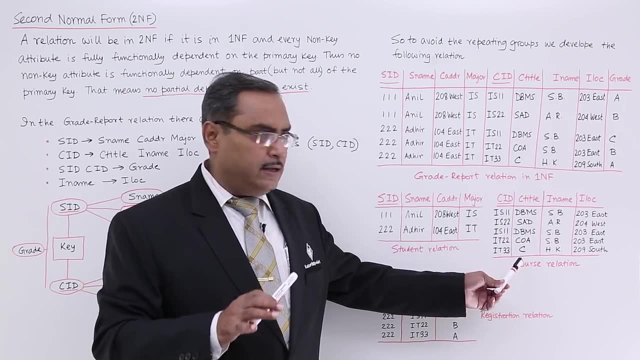 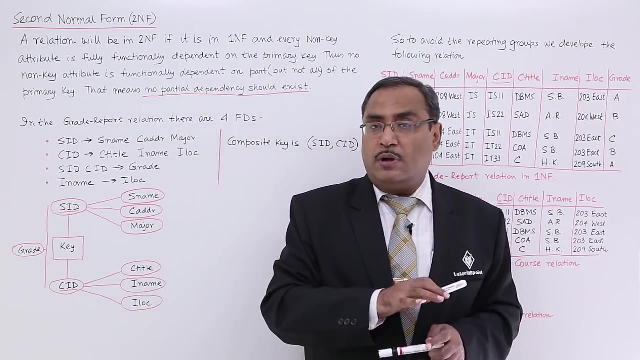 happen, the student tuple will get deleted from the student relation, respective registration relation. we can do the deletion accordingly, but the course will remain persisting in the course relation. the course is not getting deleted with the faculty and instructor details and all. so we have resolved all the insertion, deletion, updation anomalies which we had in our earlier case when the deletion 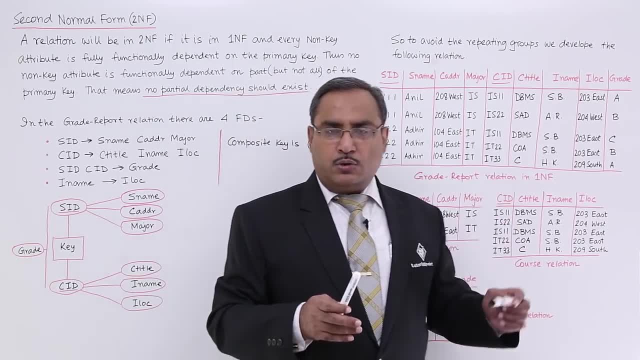 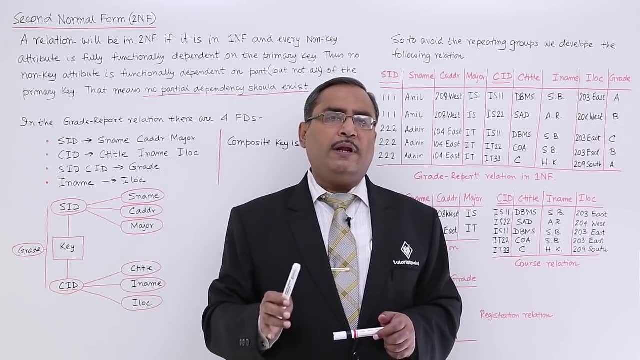 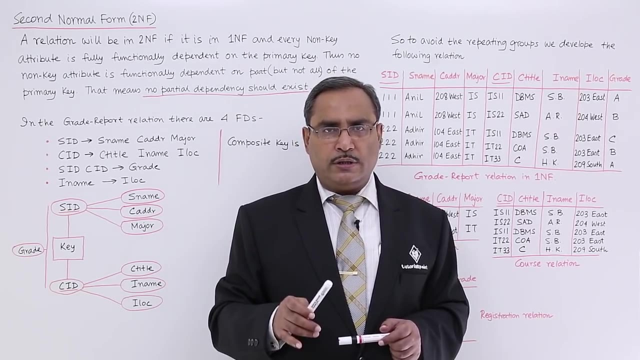 was not in 2nf, was only in 1nf. so i think now the conception is getting clear to you that how this 2nf is resolving all these three anomalies. in the next video we will be going for 3nf. please watch all of them because all those videos are in continuation. thanks for watching this. 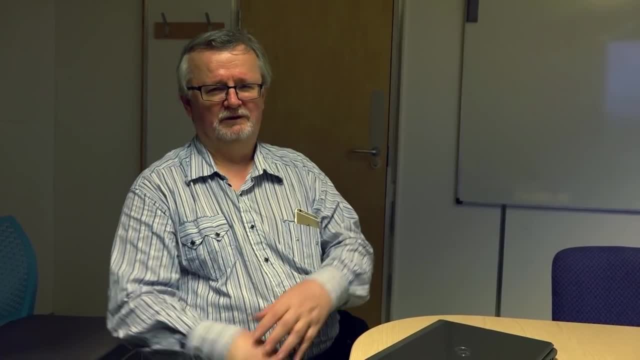 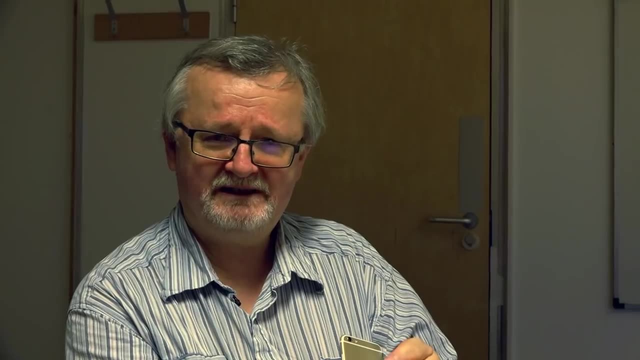 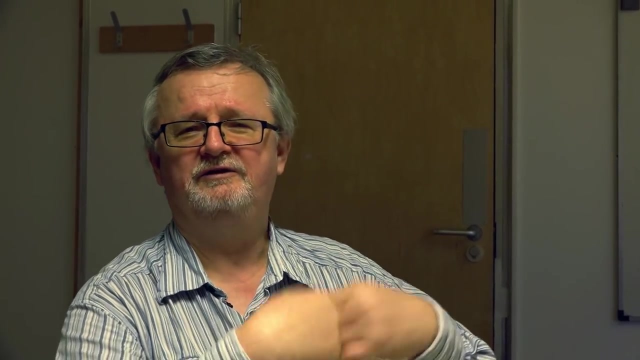 Functional programming is essentially a kind of programming where functions don't have side effects. So what does it mean? When you call a function, you give it some inputs and it will return some output, And that's all that it does. It doesn't modify the inputs, It doesn't do something on the side. 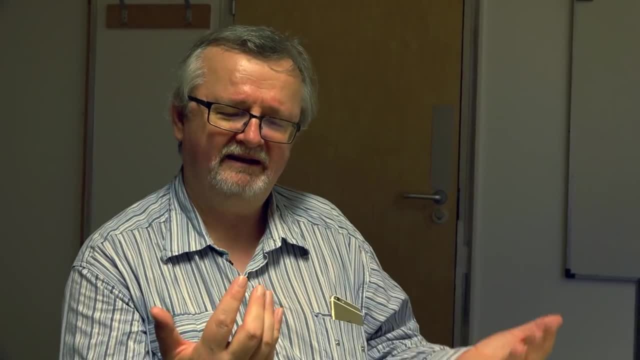 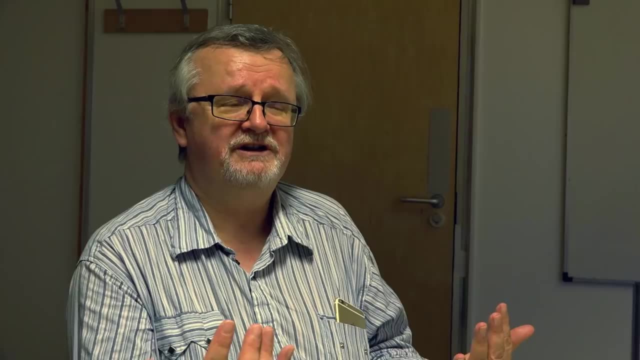 People often talk about firing the missiles. It can't do that. The entire behaviour of the function you can see by looking at what the inputs were and what the output was that was generated. And if you program in that style, then functions are you know. you know a lot about their behaviour.